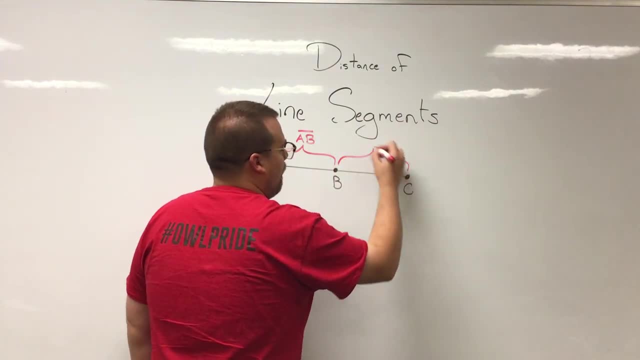 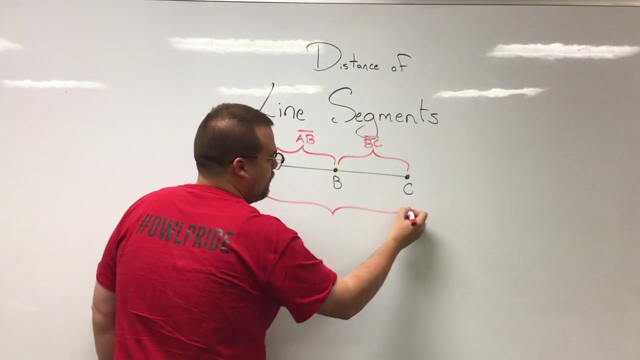 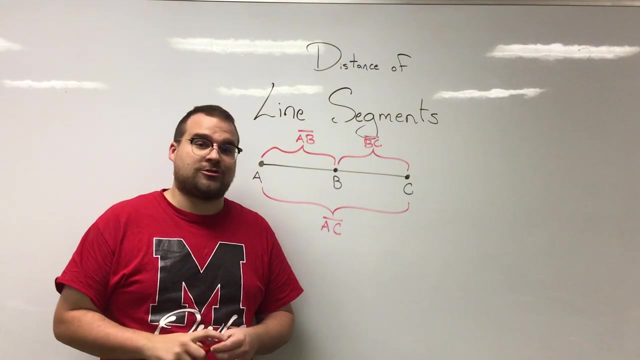 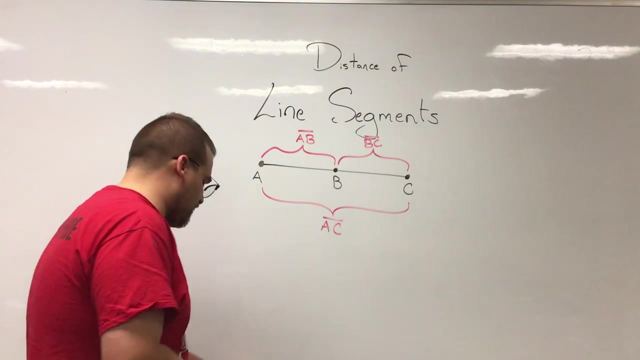 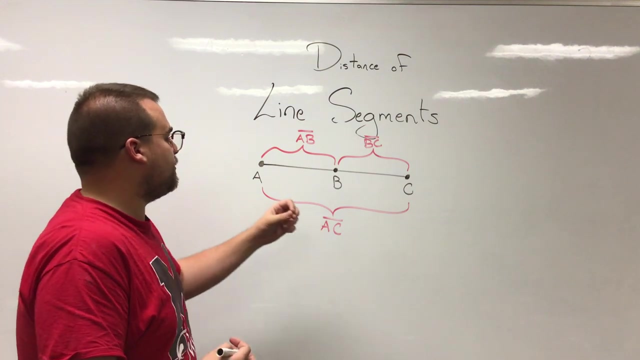 We have line segment BC right here, And then this whole thing is line segment AC. Now we can actually construct some theoretical equations using these line segments. You know that may sound weird, but we can quite literally write an equation based on how these line segments relate to each other. Here's what. 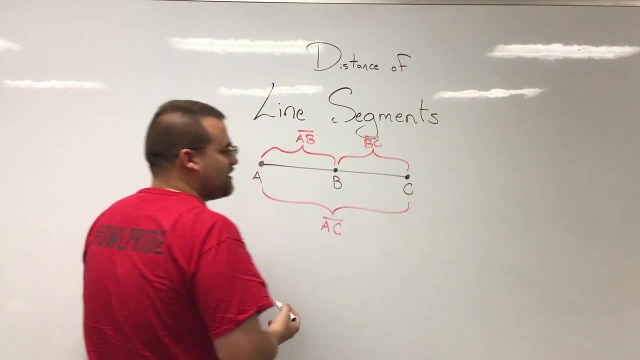 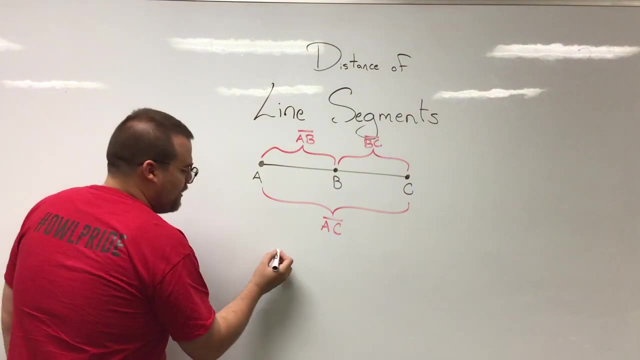 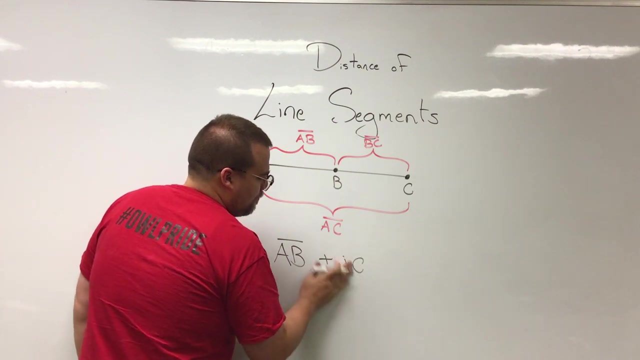 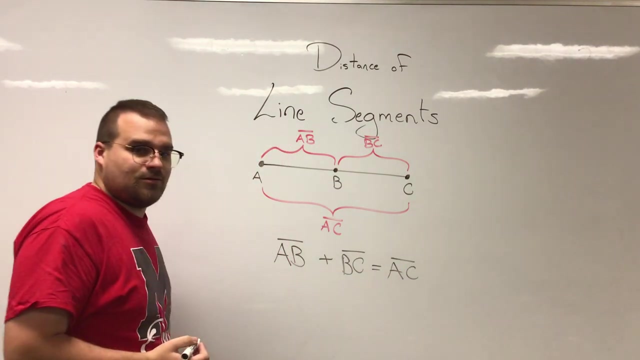 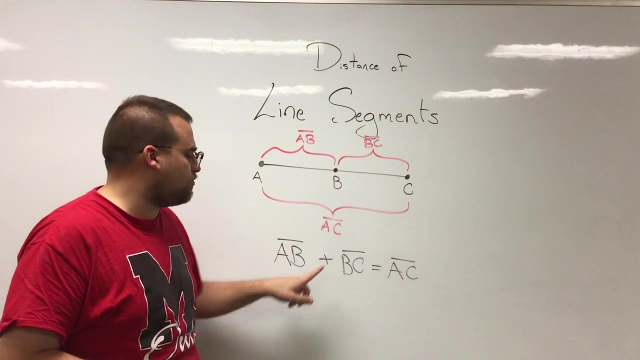 I mean, If this entire thing is A and C and it's made up of the part AB and the part BC, then couldn't we write: line segment AB plus line segment BC equals line segment BC AC. I mean, that makes sense, right? This larger segment is made up of these two smaller ones. 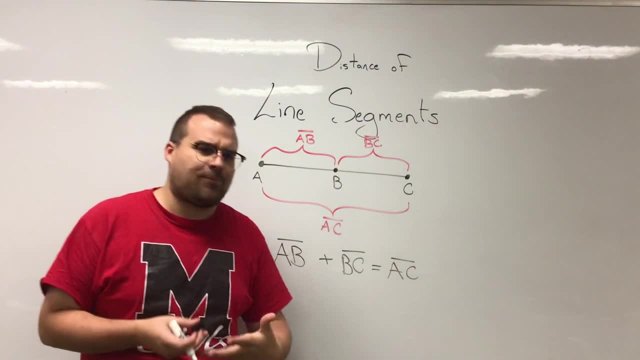 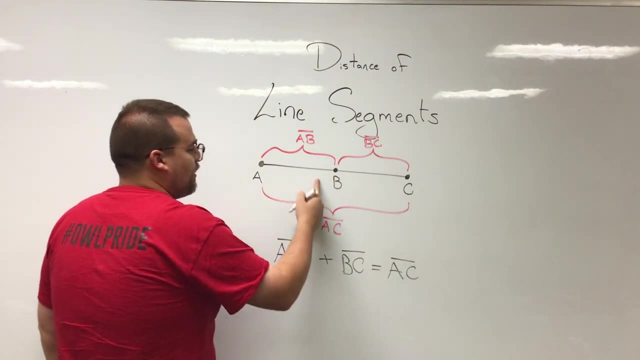 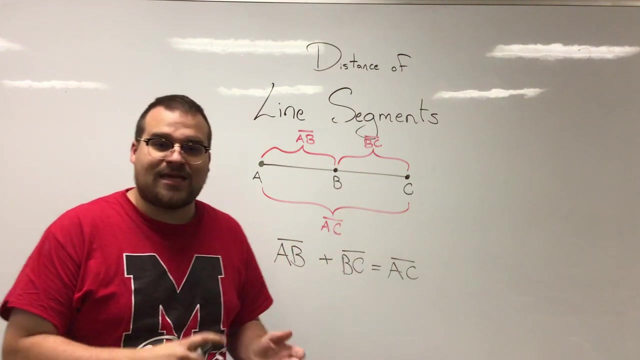 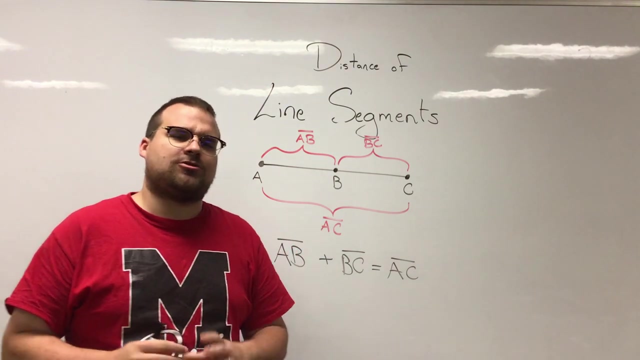 together. Now you can actually extrapolate that and make some other equations too. You could say: well, you know, if we just want to have AB, well AB is the entire thing without BC. Maybe you could do that. There's a whole lot of different ways you can do that. What I want us to do now is I want us to 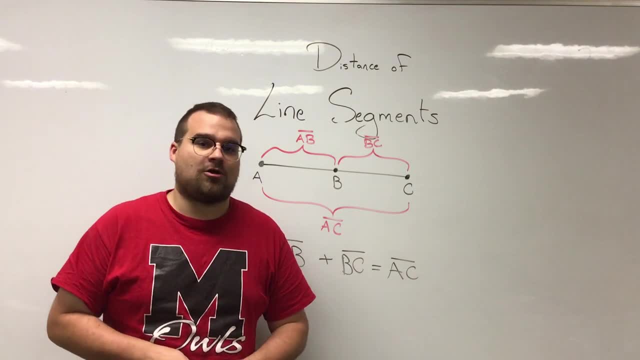 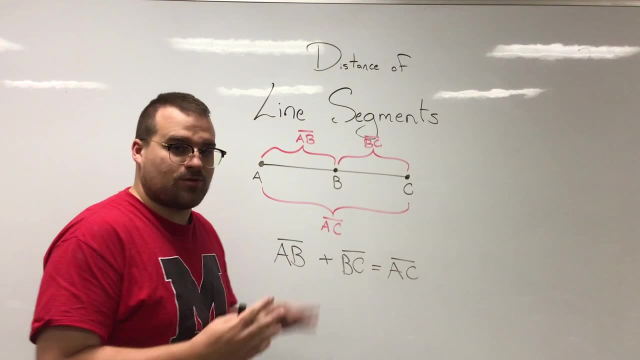 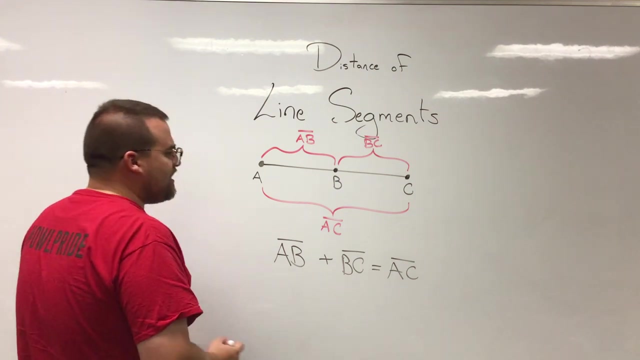 talk about a little bit of vocabulary that goes along with line segments, and then we're going to put this into use when talking about actually solving some problems that I'm going to put on the board here. So let's say that B is a midpoint. 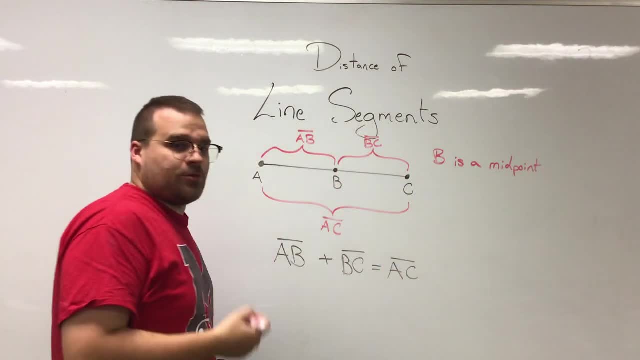 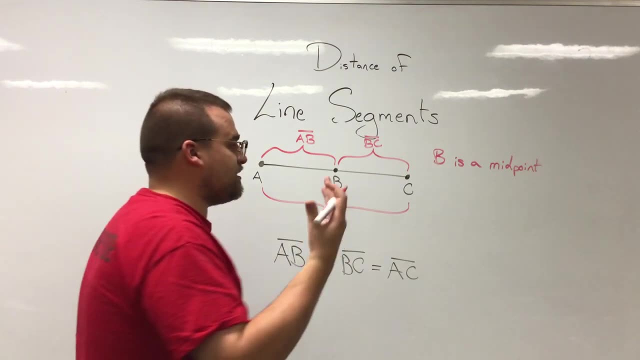 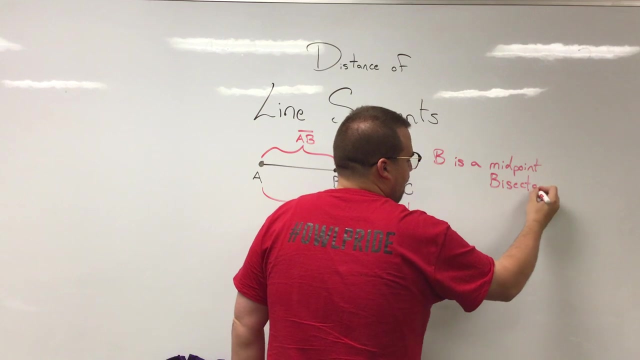 Now, midpoint is the term we're going to be talking about, but I also want to talk about a synonym for midpoint, another word that means the exact same thing that you may also hear, and that is that B bisects the line. 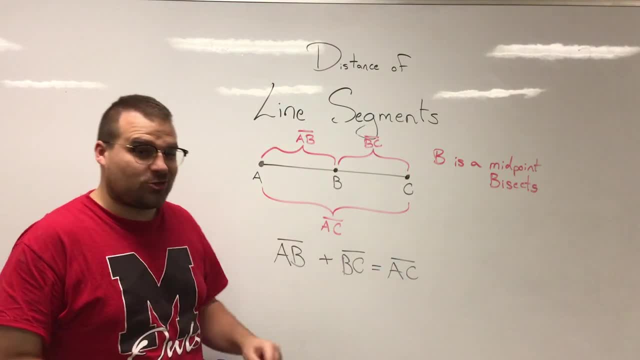 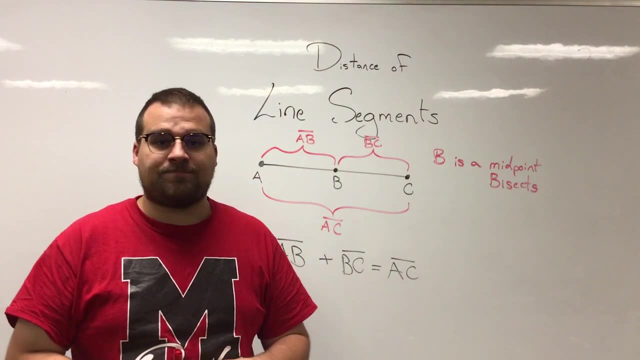 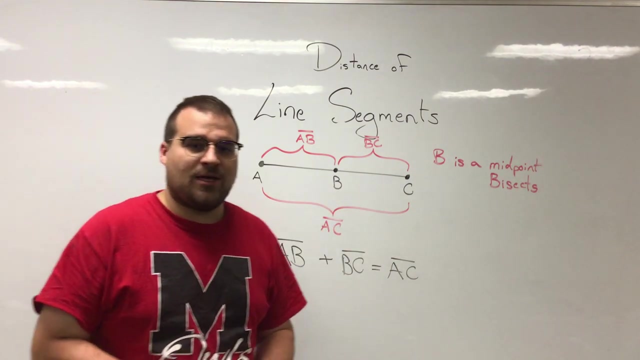 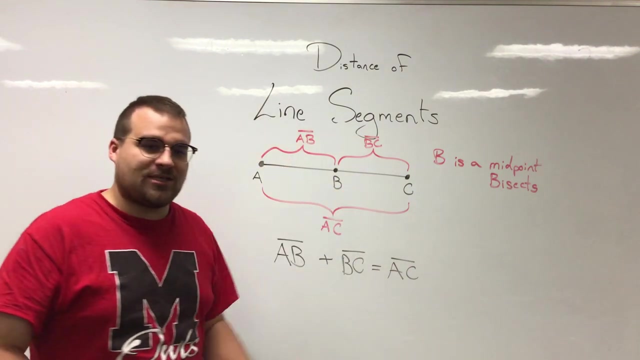 This means that B isn't just somewhere in the middle, but B is the middle, The exact center, right Now. whenever you have a midpoint, it quite literally means that it splits that line segment into equivalent halves, saying this is the exact same as this, at least in terms of distance or size. 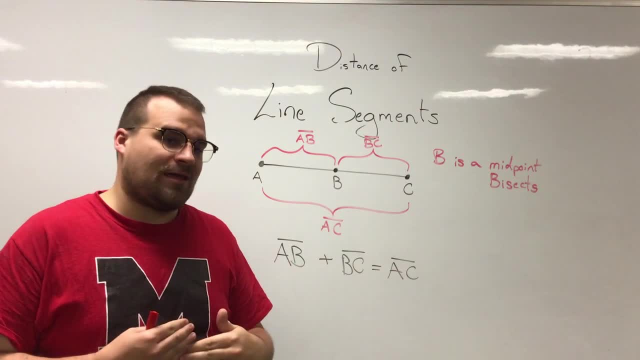 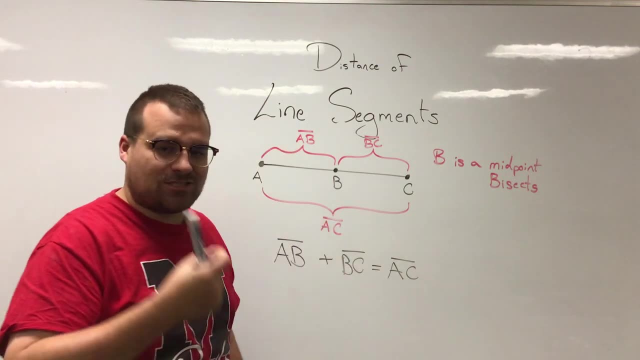 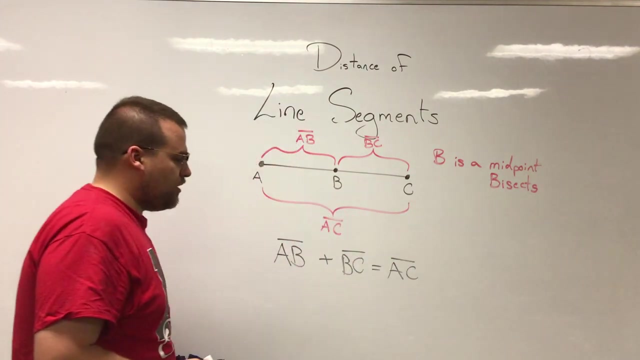 So that is what a conclusion that we can draw. whenever we hear something like B is a midpoint or B bisects the segment. Again, those two mean the exact same thing. So if we understood that this is true, then maybe this isn't the only kind of equation we could create. 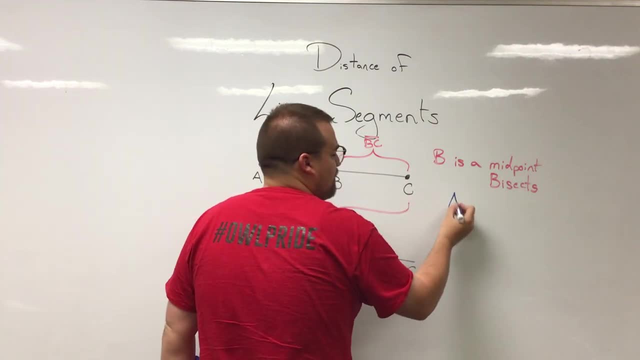 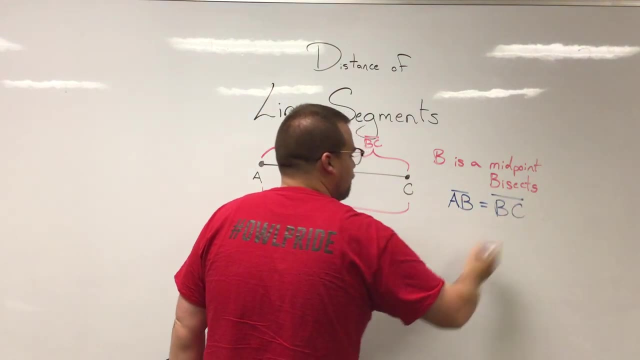 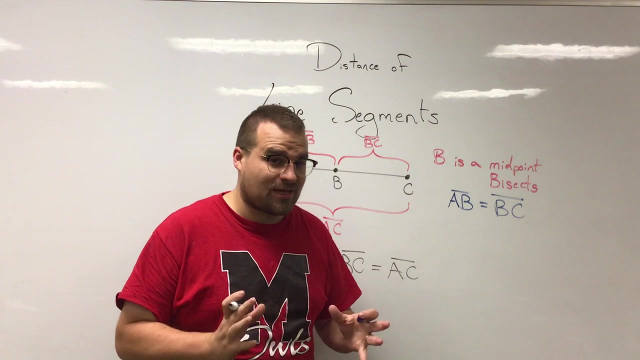 Maybe we could also say: line segment AB is equal to line segment BC. Now, if we didn't know that B was the midpoint, could we make that statement? Could we say this in all cases? No, We have to know that B is the midpoint in order to say that. 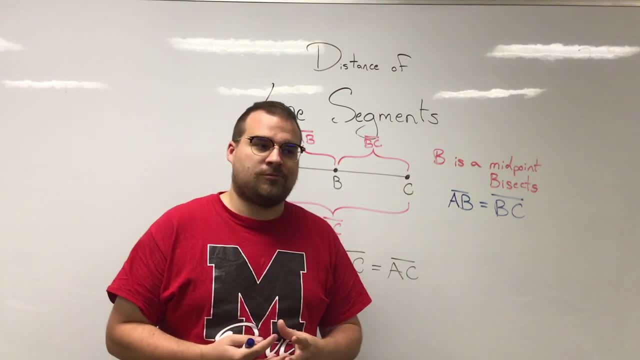 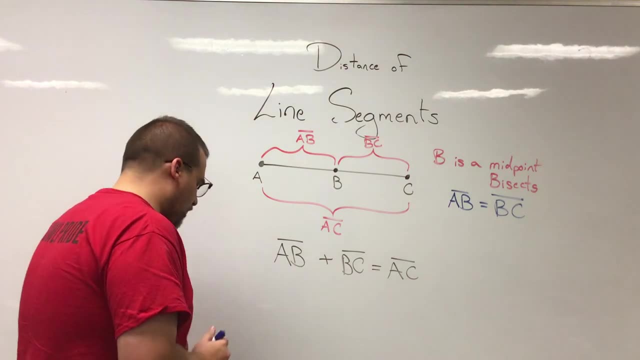 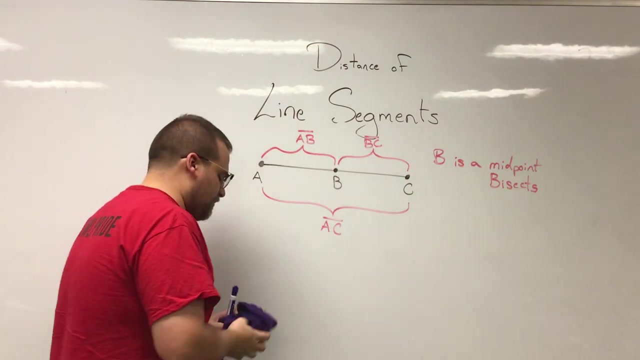 But when it is, that's an important thing to remember. Of course, the letters might be different, but you can make them match whatever problem you're working with. Alright, let's get into an actual mathematical problem. We're going to keep in mind that B is the midpoint and B is a bisector. 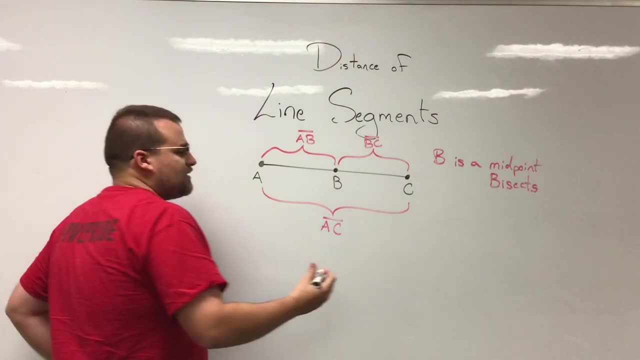 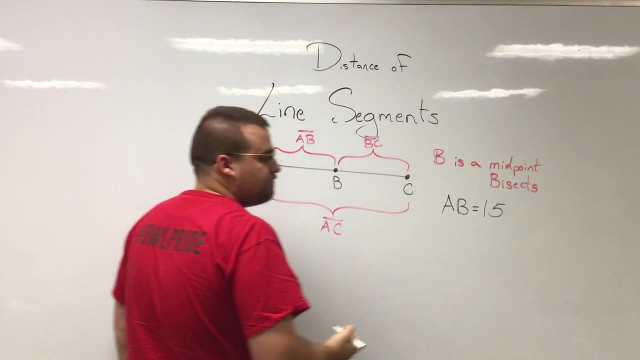 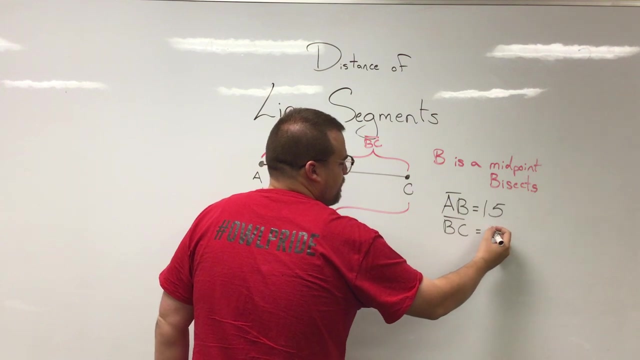 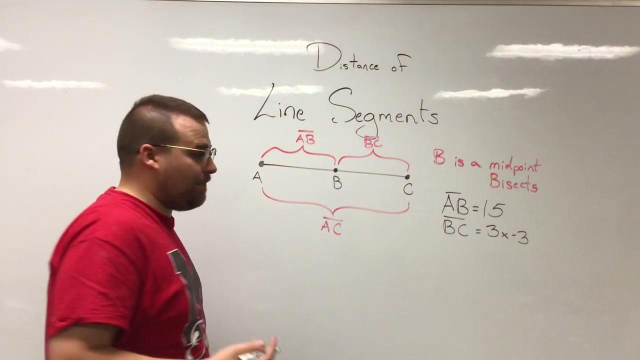 So I'm going to leave that just like it is. Let's say AB is equal to 15 units, and then BC is equal to 3X minus 3 units, And the problem might want you to say: well, what is X? 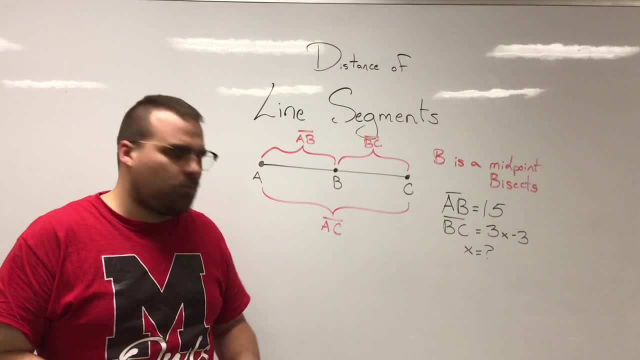 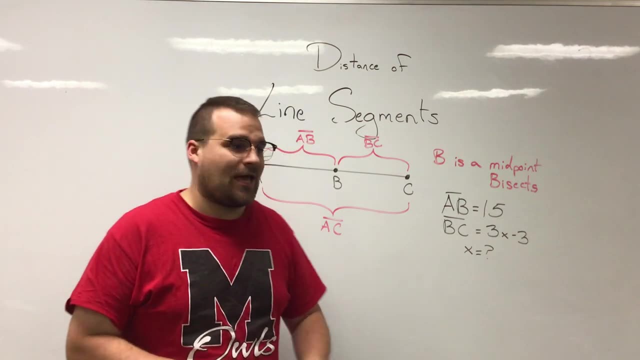 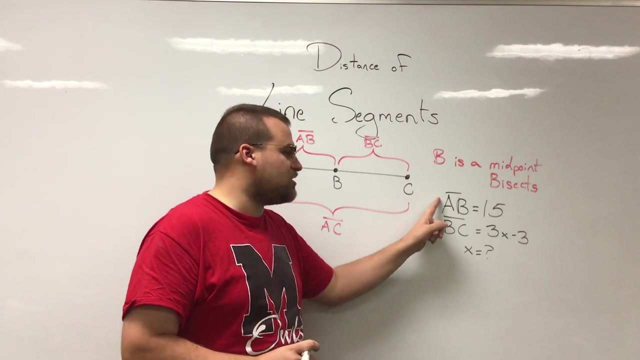 How would we do a problem like that? Well, we want to ask ourselves: with the information we have- we know what AB and BC are, and we know that B is a midpoint- Can we form an equation that will relate these two segments together? 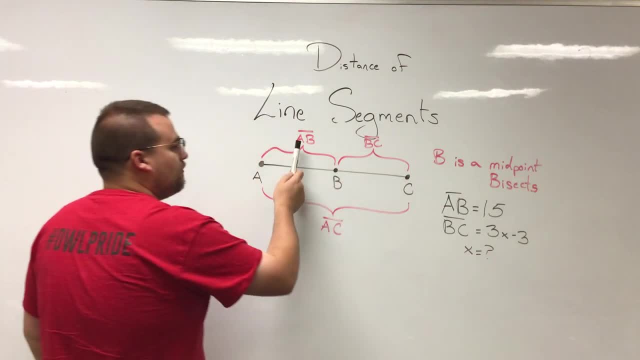 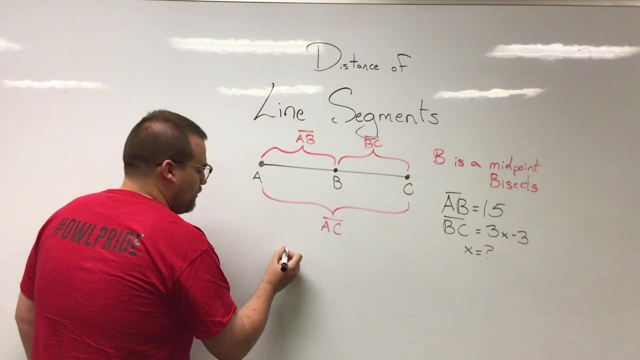 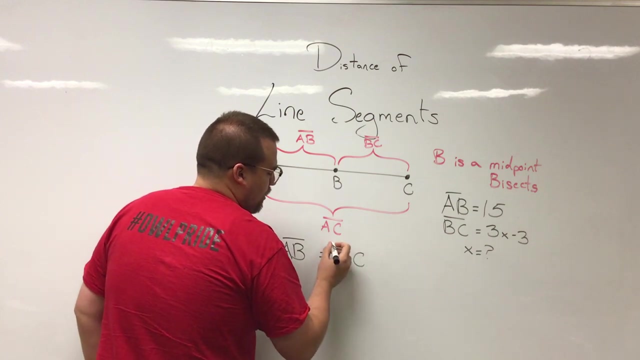 Well, we said earlier, if we know this is a midpoint, then we know these are equal. So I'm going to take that thought, that idea, and turn it into an equation. That's an important skill that we need, What we have to kind of master a bit or at least become comfortable with in geometry. 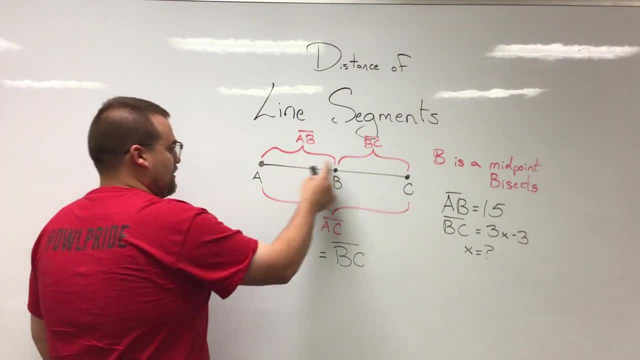 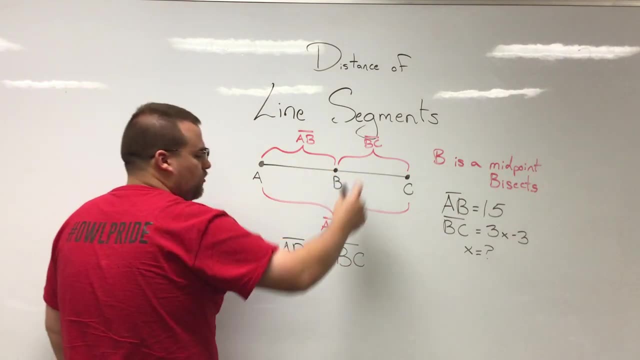 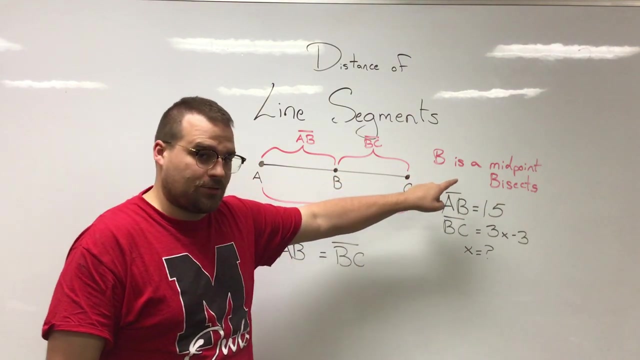 is making sure we can take that concept, that thought that these are equal, or whatever thought you may have, and write an equation with that information: AB equals BC. Now that I've created this equation based on my given information, I can substitute in what they're equal to: 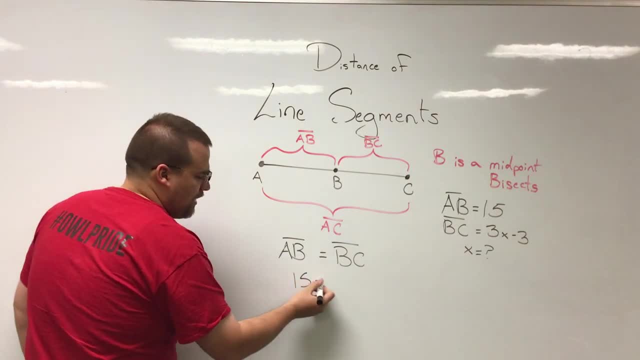 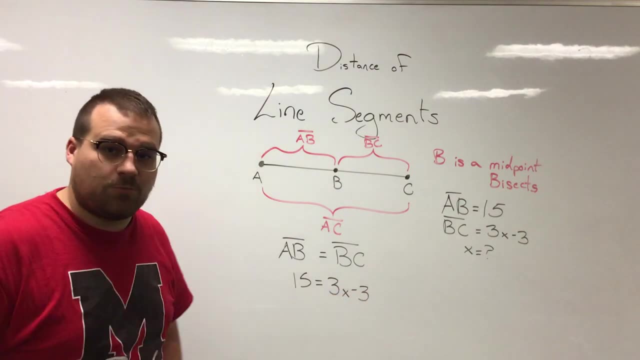 AB, Well, that's C, That's 15. And BC, that's 3X minus 3.. Now I can solve this just like we would an algebra problem. Add 3 to this side to get those to cancel out. 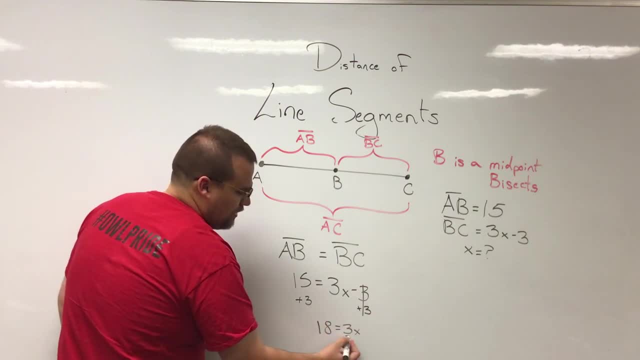 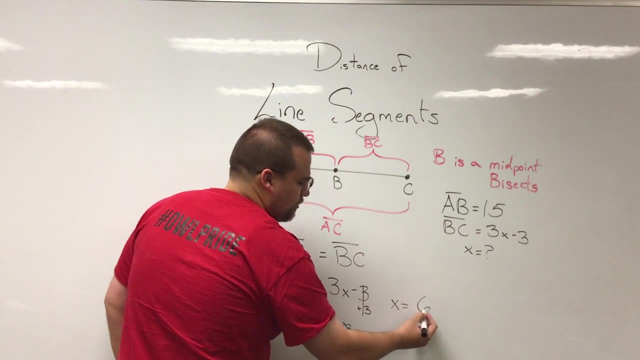 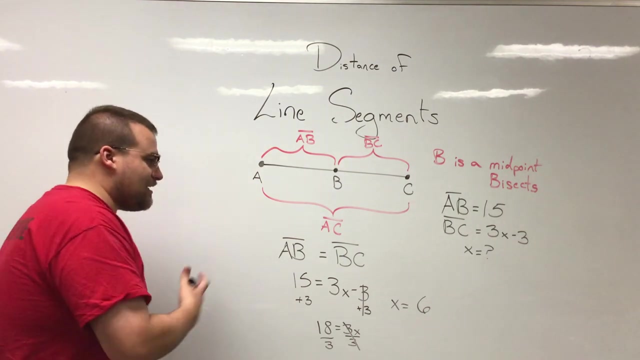 Get 18 equals 3X, And then get X on its own by dividing by 3.. And guess what? X equals 18 divided by 3, or X equals 6.. There we go, We found X. Now what if this wanted us to take it one step farther? 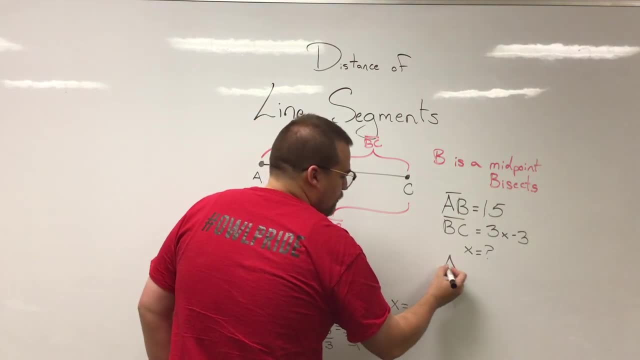 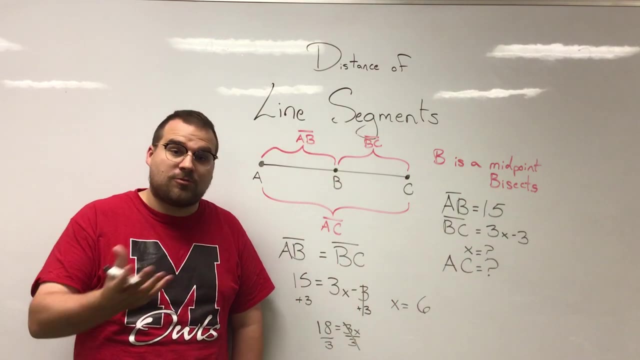 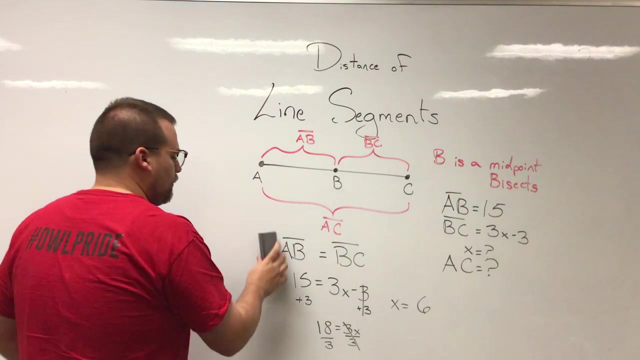 And it wanted to say: well, what is AC equal to? Could we figure that out? We could. We actually have multiple ways of figuring that out. Here's one way we could think about it. We could think with the equation that we made earlier. 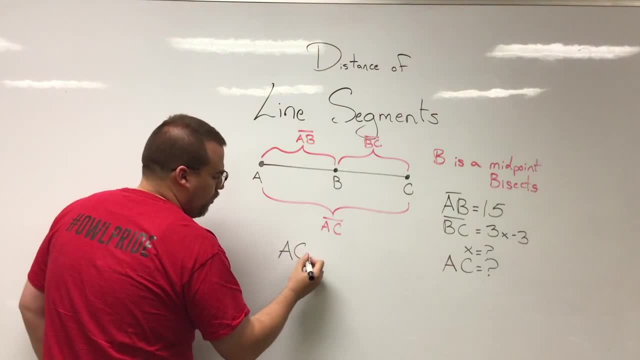 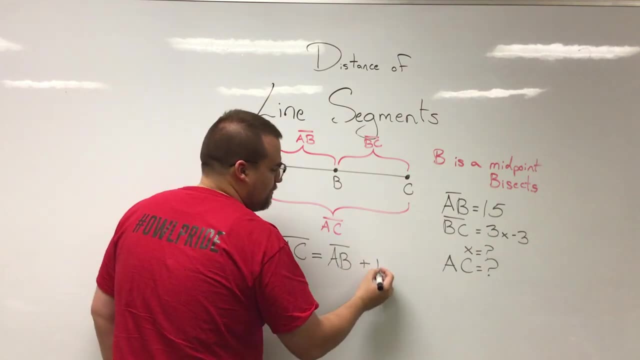 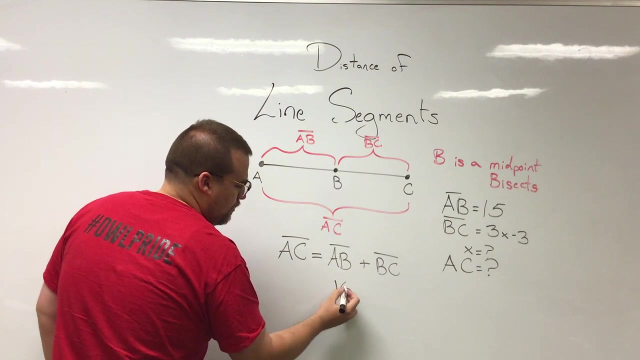 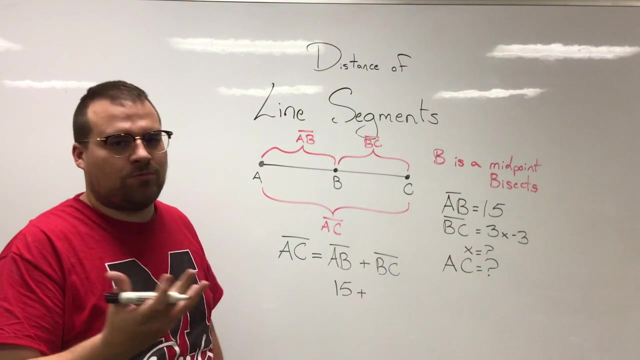 that AC as a whole is made up of AB and BC. Okay, Now we know AB is 15.. And I mean we know BC was 3X minus 3, but does that really help us? No, But what we could do now that we know X is 6, we figured that out already. 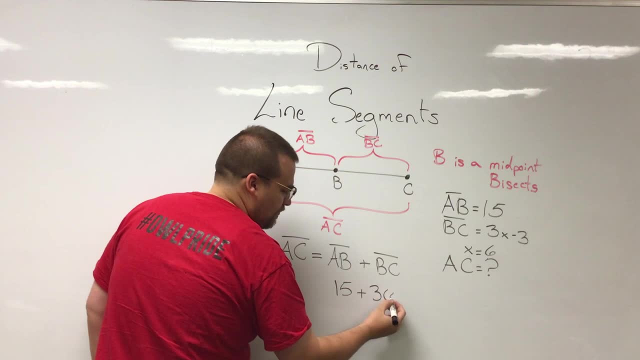 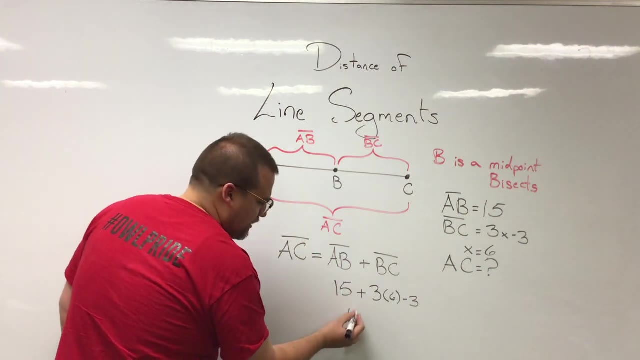 is, we could write this with 6 involved. So 15 plus 3 times 6 minus 3.. Well, order of operations tells us we've got to do 3 times 6 first, so that's 18.. So 15 plus 18,, that's 33.. 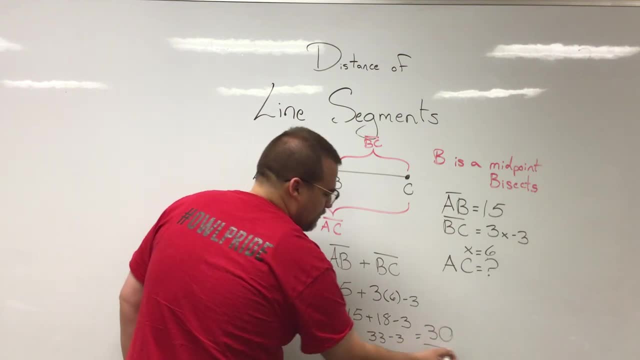 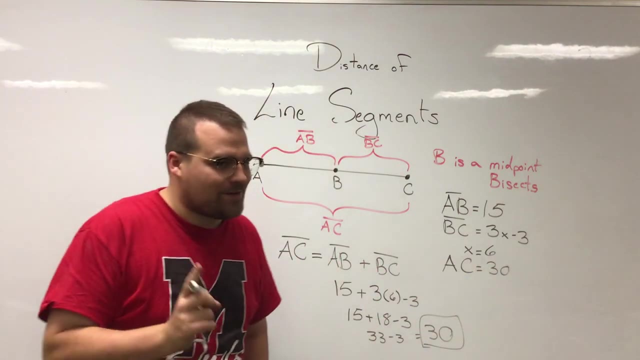 And 33 minus 3, guess what? That's 30. That's our value of AC. Now you may be thinking to yourself: there was a lot easier. There was a lot easier way to go about that. There was a lot easier way to figure that out. 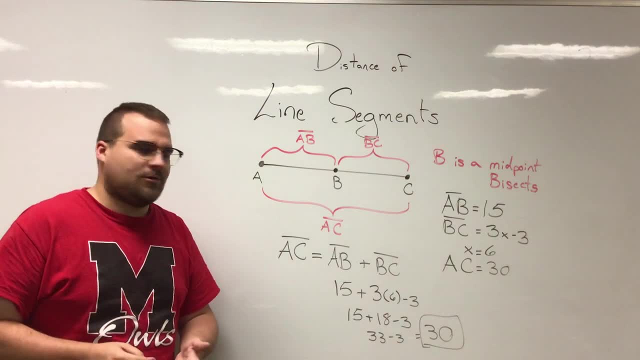 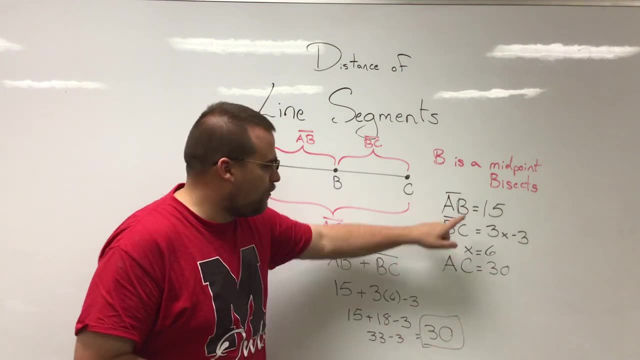 I mean that worked, But we could have done it a little easier. And you're right. If we know B is a midpoint, B cuts it in two equal halves. if we know the length of one of them, then guess what. 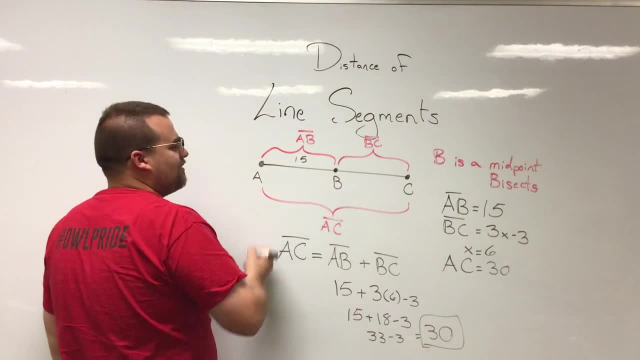 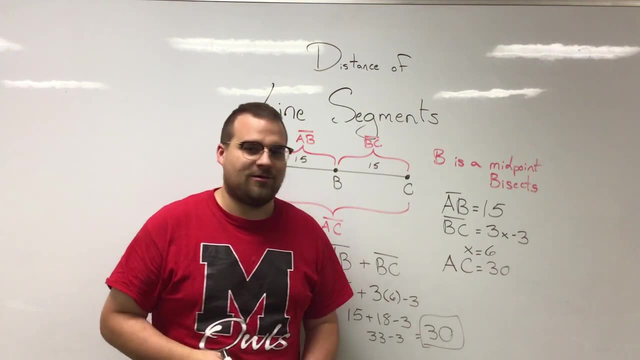 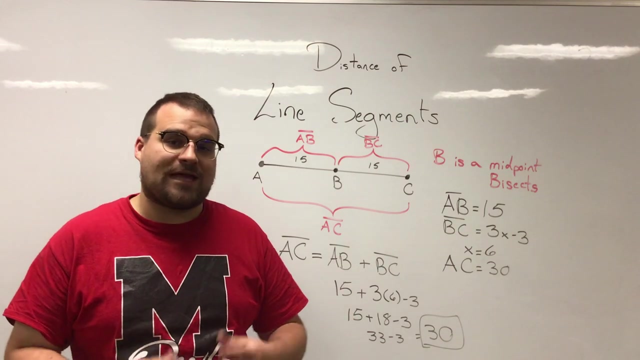 We know the length of both, right. If we know this is 15, and that's a midpoint, we automatically know that's 15,, so the whole thing must be 30. Exactly Now. like I said before, there's so many different ways you can have problems like this. 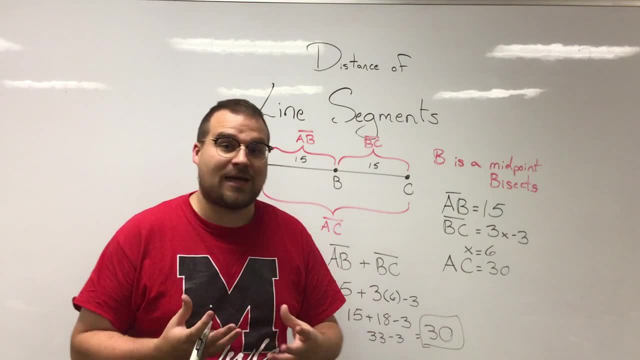 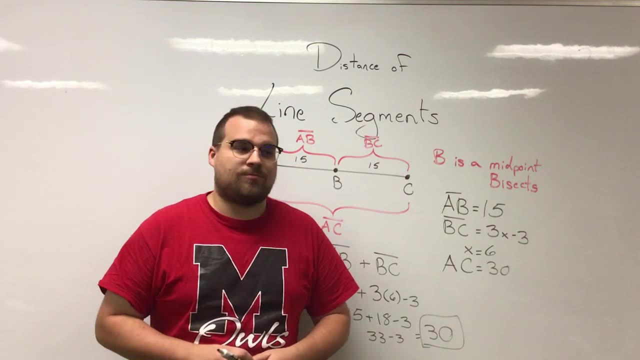 So many different bits of given information and so many different ways line segments can be constructed- Honestly, a lot more ways than you probably would expect. We can't cover those all here and probably not every question you may have is going to be able to be answered here. 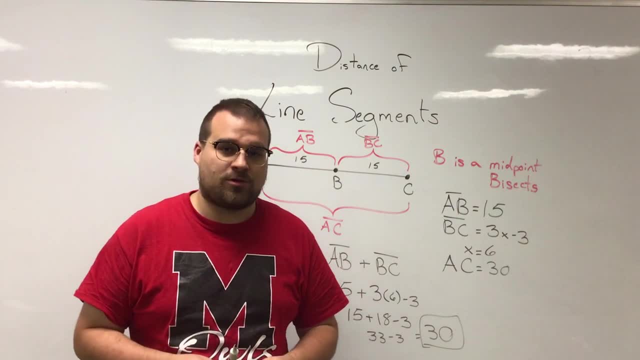 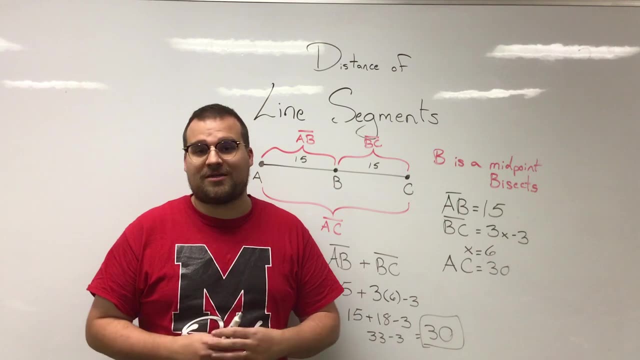 But we are going to have an additional video going over some other examples that I think may help us out a bit. If you have any specific questions, please drop them in the comments below and I'll do my best to get back to you and help out with those. Otherwise, thanks for watching, guys, and I'll see you next time. 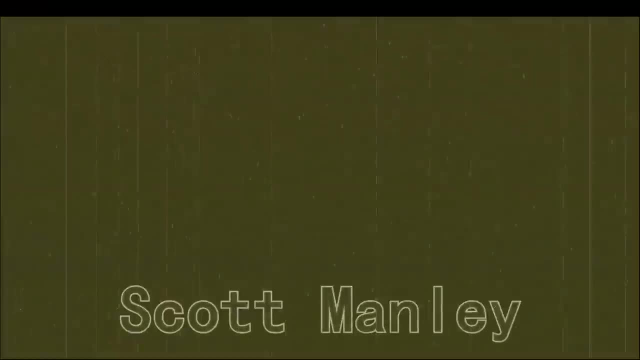 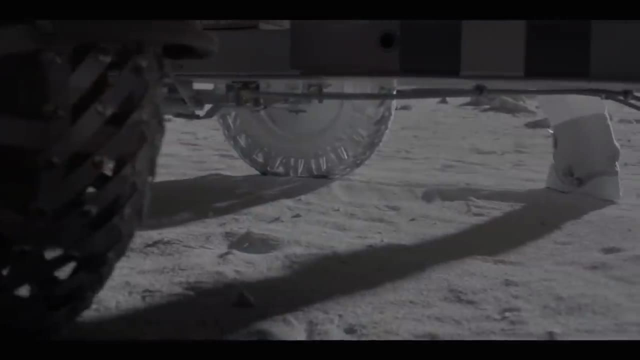 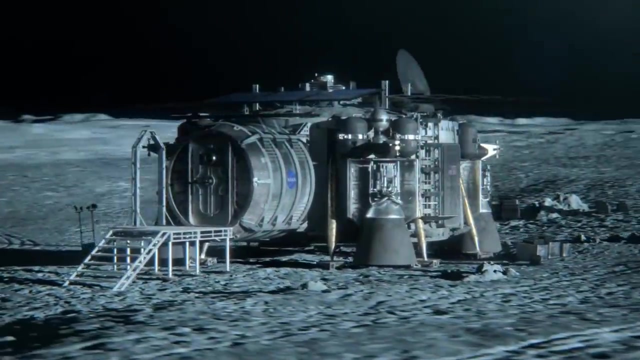 Hello, it's Scott Manley here. The TV show for all mankind follows an alternate history of the space race, A history where Alexei Leonov becomes the first man on the moon and the US goes all in on developing the Apollo program into something bigger and better. Season one ends with a base. 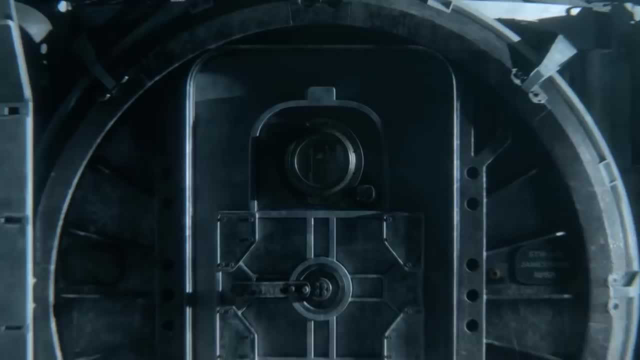 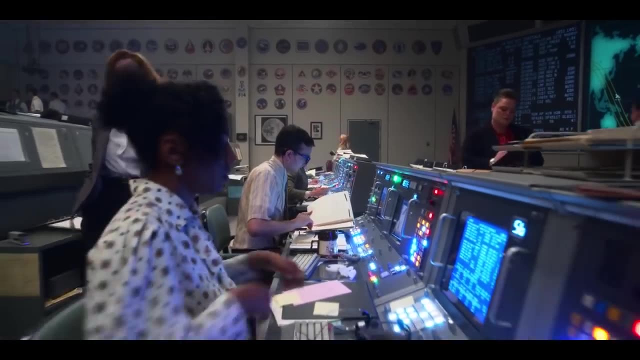 on the lunar south pole harvesting water, trapped in the permanent shadows of Shackleton crater. And now the trailer for season two has dropped and time has moved forward to the 1980s, where we see Reagan giving speeches and squads of astronauts with assault rifles. But the thing I want to talk-